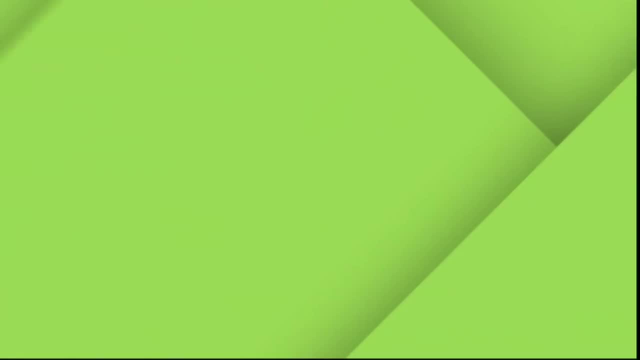 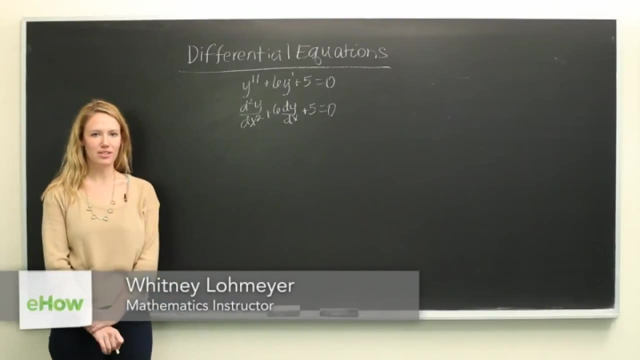 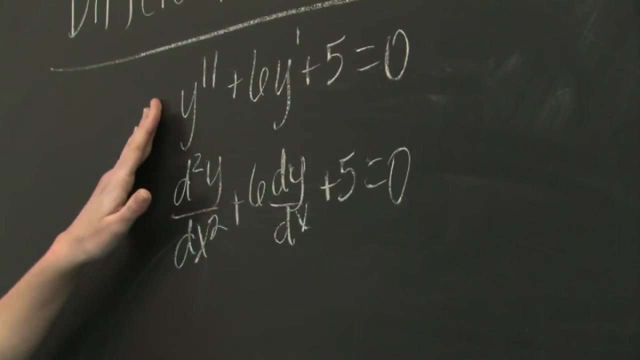 Hello, my name is Whitney and this video is going to go over differential equations for beginners. So, starting with the basics, we have a differential equation written on the board: Y, double prime plus 6y plus 5 equals 0.. This can also be rewritten as the second. 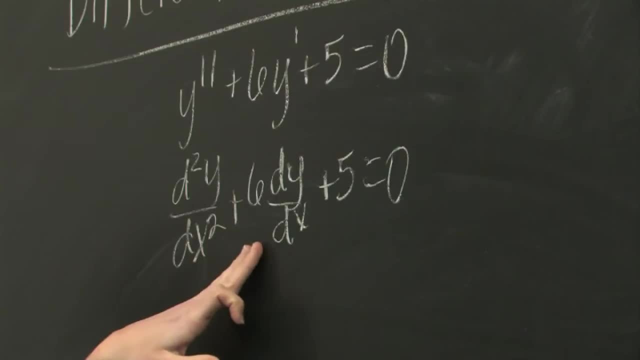 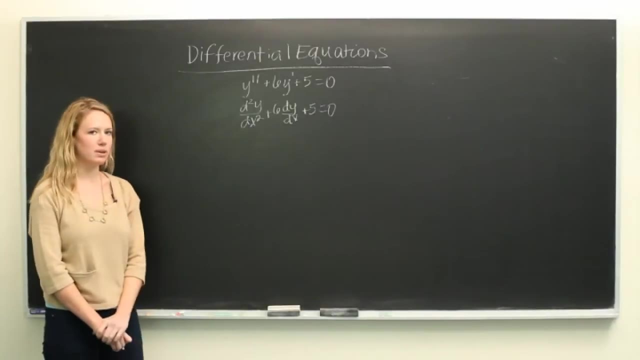 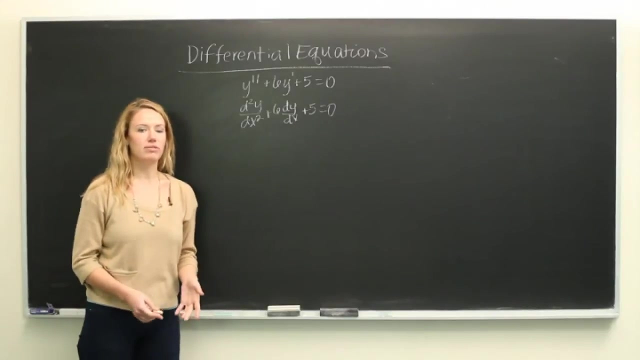 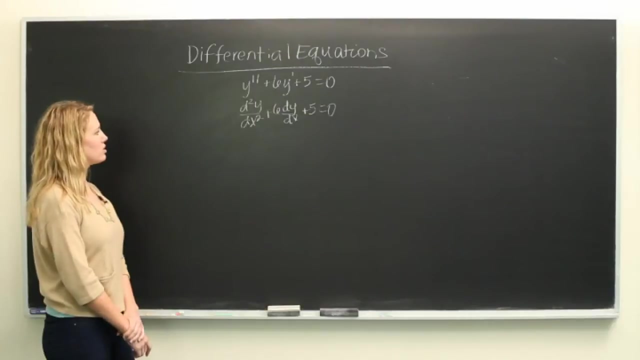 differential of y plus 6 times the derivative of y plus 5 is equal to 0.. Now the first step in solving our differential equation, or writing it as the form y is equal to the sum or difference of a few terms, is to figure out the roots. Now, to do this, we're going to write our equation. 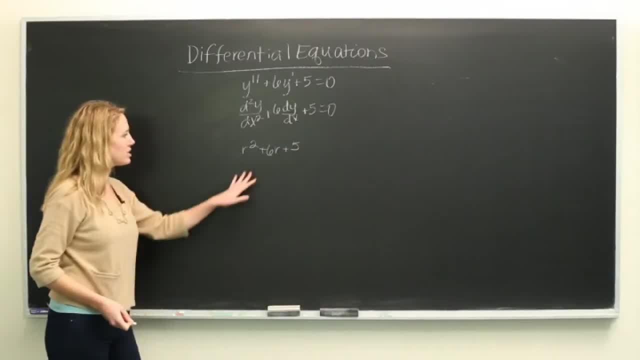 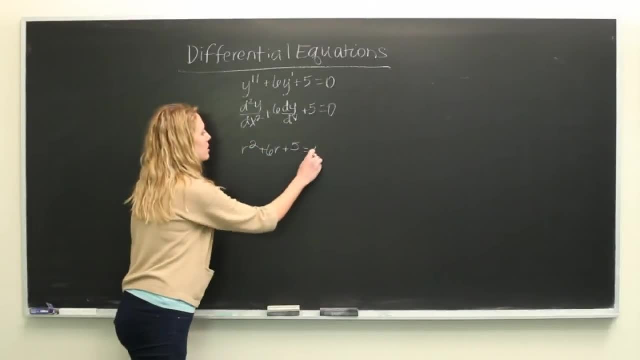 in a bit We're going to write our equation in a bit of a different form, where r takes the place of the first derivative. So if you have r squared, that simply means second derivative, And we're going to unfoil this. so factor this trinomial. Again, both signs are positive. 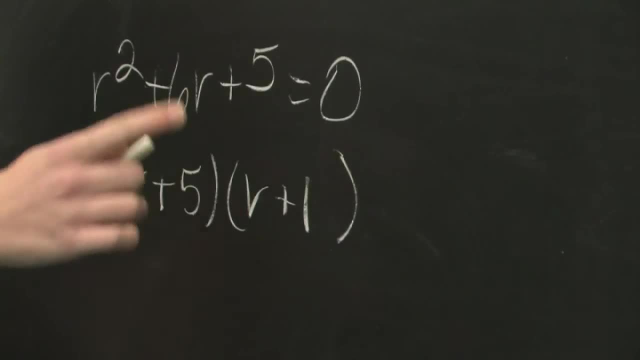 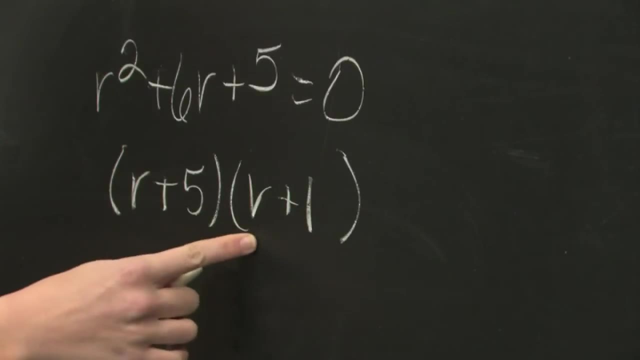 since the second sign is plus, that means both signs will be the same and it takes the sign of the first term. It'll be it. We know that r squared is equal to r times r and that 5 times 1 will give us 5. and when? 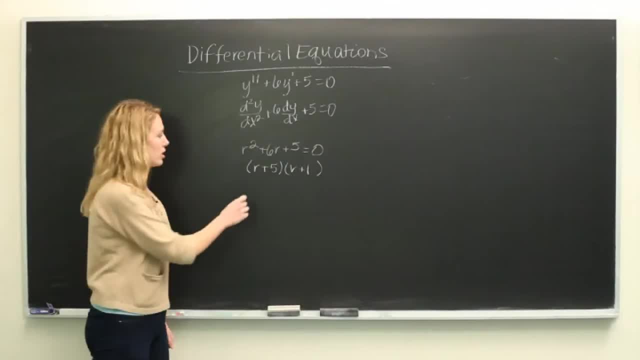 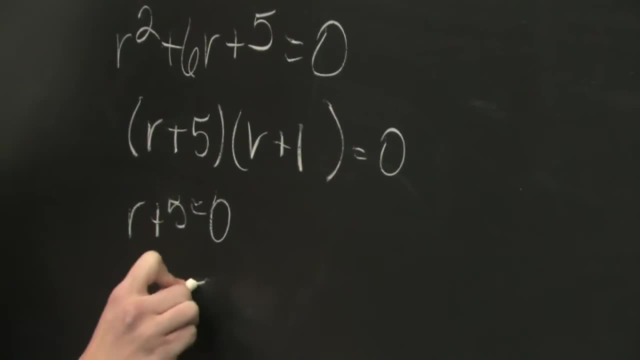 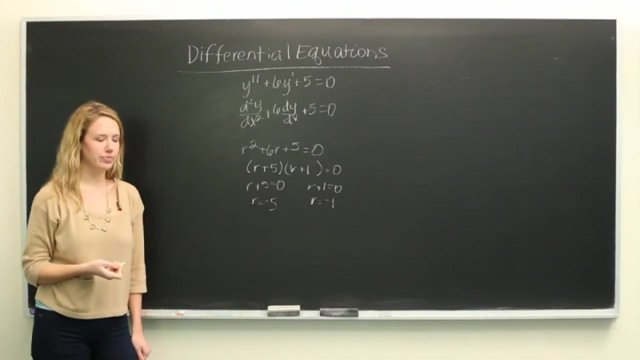 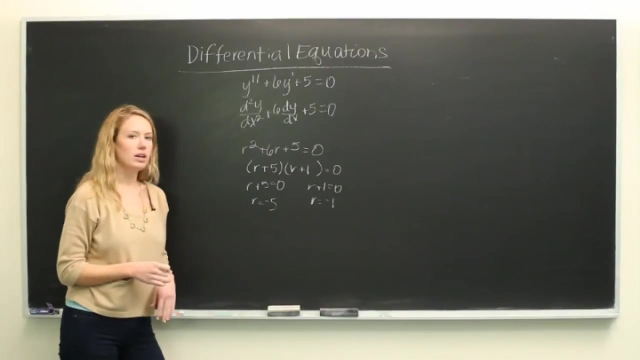 we add them, it will give us 6.. So our roots are equal to minus 5.. and minus one taught with a group reference. So since these values are real, So since these values are real numbers that are not the same, This is called something case 1.. So a case 1. 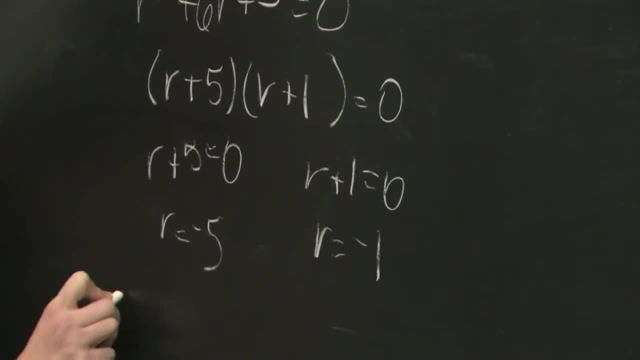 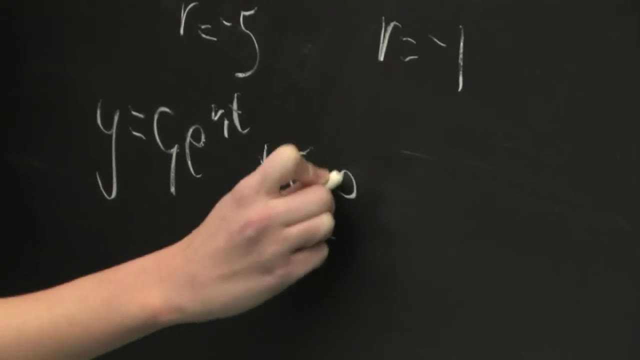 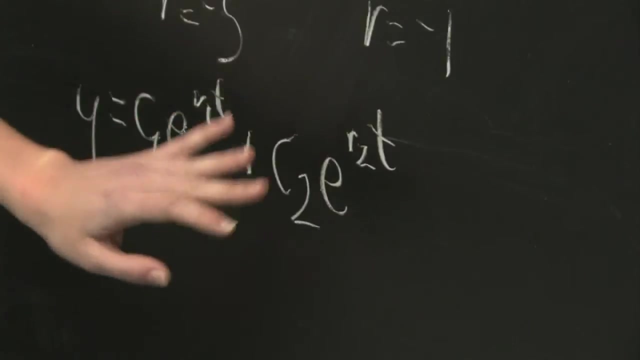 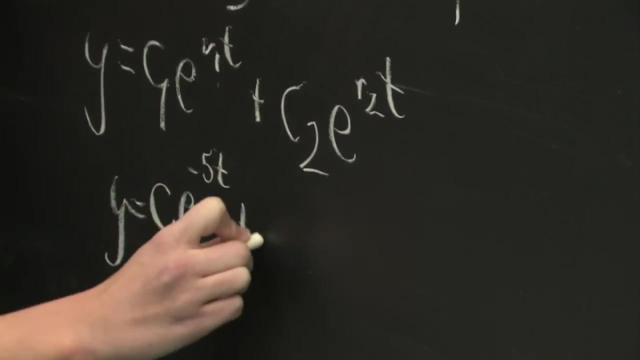 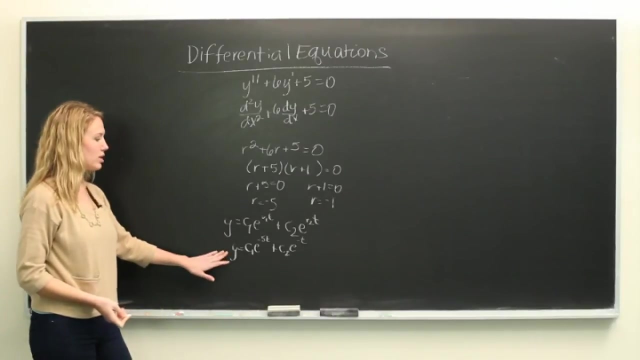 differential equation will follow the form: y is equal to c1 e to the r1 t, plus c2 e to the r2 t. And to solve our differential equation all we need to do is plug in for r. So it's okay to leave the equation here. You have solved your.